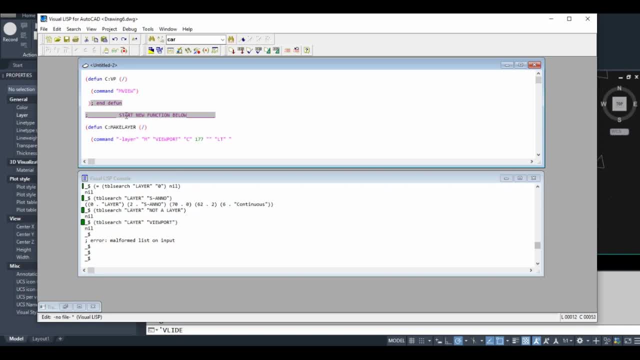 prompt at this point you'd hit LT for line type. I want it to be phantom 2.. What was our last thing? It was a plot or no plot. So p for plot, No plot. And then we hit enter one more time to exit the command. 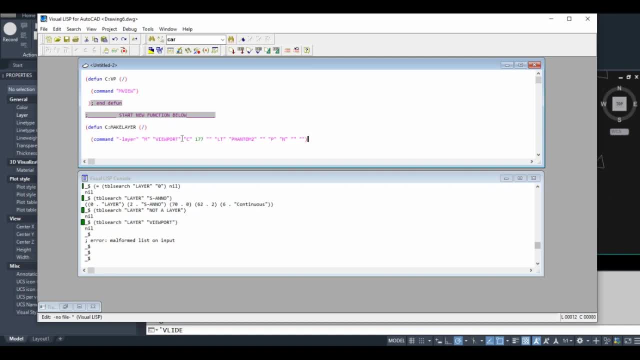 So, just in case I made a mistake, let's test this out, Make sure that works. So, just in case I made a mistake, let's test this out, Make sure that works. And sure enough it did. So I'm going to show you another function now. It's called the table search function. 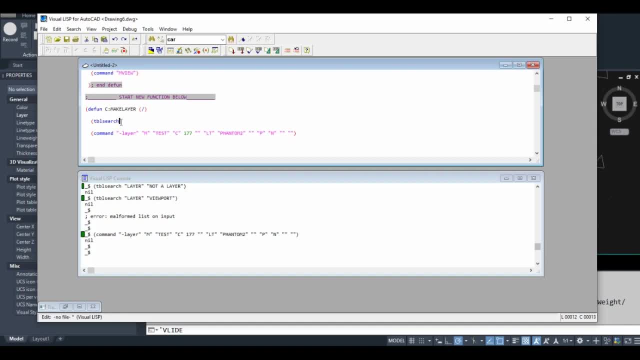 Anytime I introduce a new function, if you want to know more about it, go to Google and search the function and autolisp together, of course. Usually an Autodesk help page comes up which is very descriptive, and some other resources as well as well, like message form. 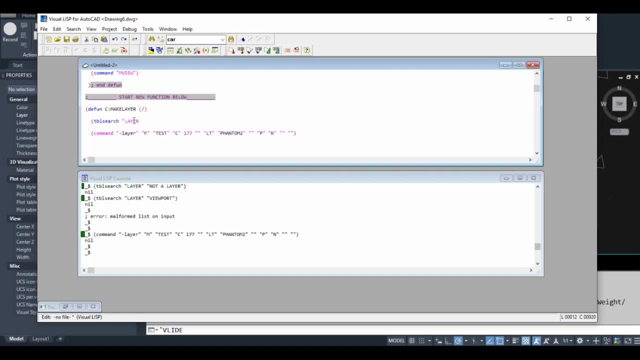 Basically, the table search function searches the various AutoCAD tables. There's one for layers, one for line types. I'm not going to get too far into it in this beginner tutorial, but all this is doing is it's searching for our layer. You can search for any layer that's in the drawing. Basically, we're trying to see if this layer exists or not. 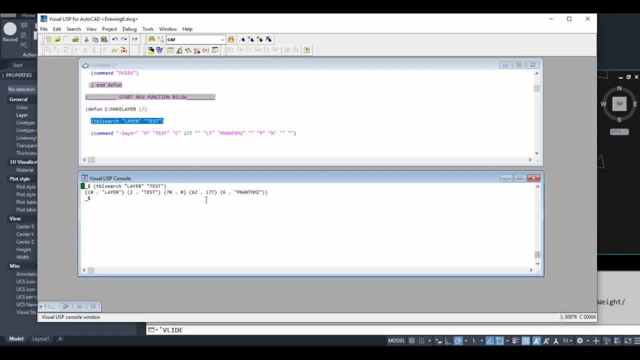 Let's put it into our console. This is a table search function. You can search for any layer that's in the drawing. Basically, we're trying to see if this layer exists or not. Let's put it into our console. This is a table search function. You can search for any layer that's in the drawing. Basically, we're trying to see if this layer exists or not. Let's put it into our console. 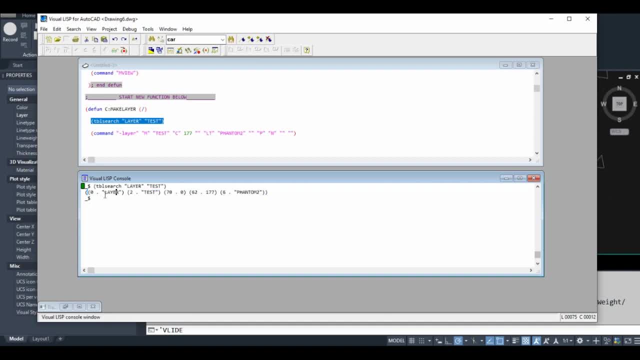 This is a table search function. You can search for any layer that's in the drawing. Basically, we're trying to see if this layer exists or not. Let's put it into our console. This is an entity list, Not something I want to get into in this tutorial, but for now, just imagine that this is something. 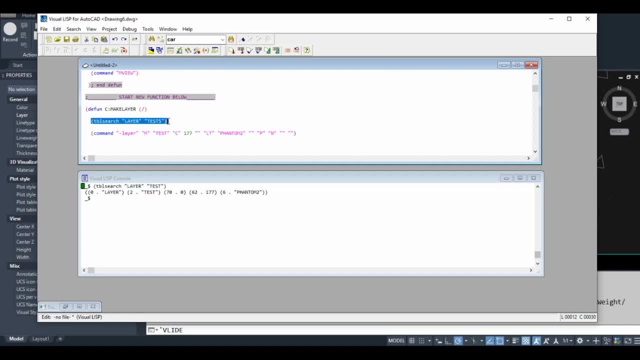 Let's put a test5.. There's no layer name. that in my drawing right now. Let's see what happens. AutoLisp returns nil. So nil, it's not zero, Nil is nothing. Think of zero as being an actual value, like zero degrees is an actual temperature. 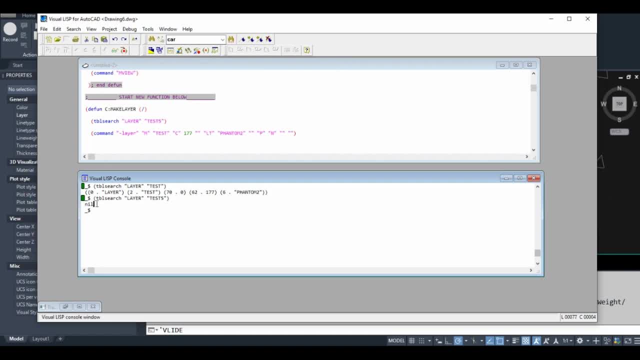 Nil is nothing. That's like the weather station is broken and not giving us any information. We can use this to our advantage, because what I want to do is make a conditional statement. What I want to tell AutoLisp is that if our layer- let's call it viewport- 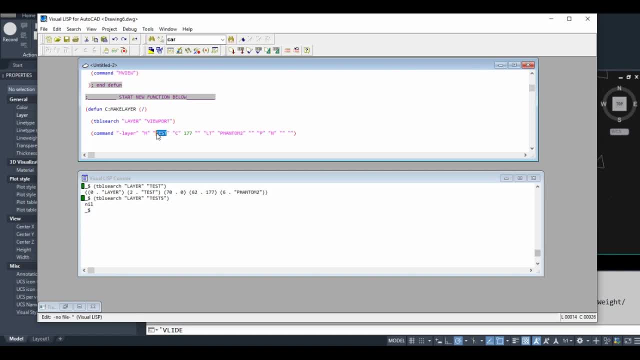 Change this to viewport here as well. I want to tell AutoLisp that if our layer doesn't exist, run this piece of code. I'm going to use the if function. I want that on the same line, I think If You'll see me add extra spaces- Spaces don't really do anything. 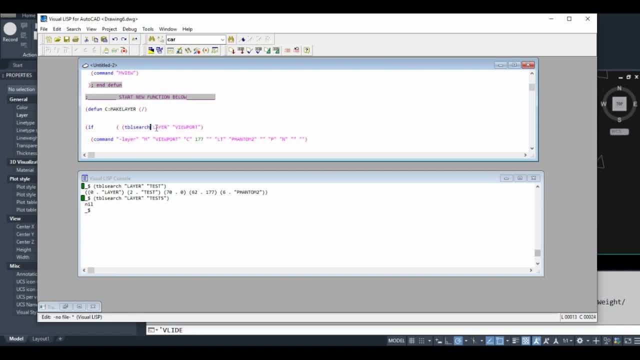 Even if I go like this, the code will work just the same. Of course you want separation. I wouldn't want to do that. Notice how that turned from blue to black. But as far as just having spaces, they don't have an impact. 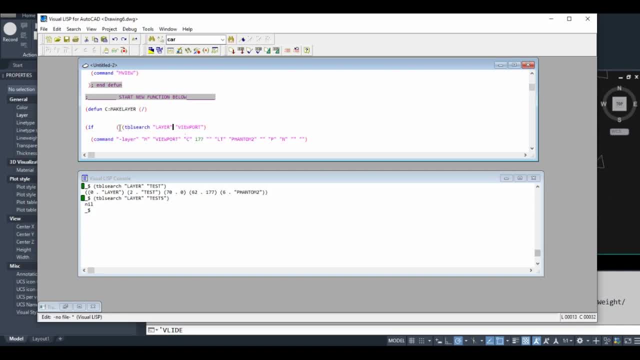 So, if So, what this is saying is: if this equals this, run this piece of code, Close off our if. Leave a little note there, just so we know that it ends More, More important as your code gets bigger. So if equals table search layer, viewport nil. 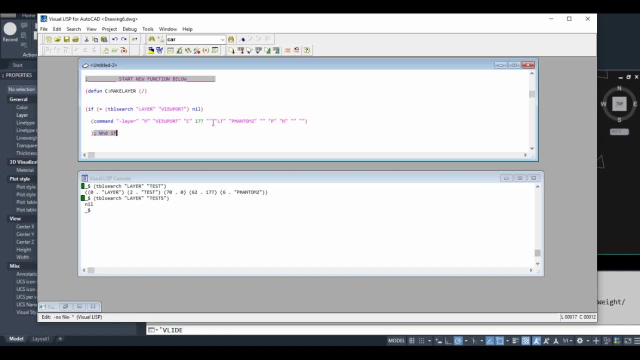 Create this code. So if statements are actually if or else, We don't have an or else statement yet. So what this code would do is, if this condition is not true, it just won't run this, It would just pass through this piece of code.